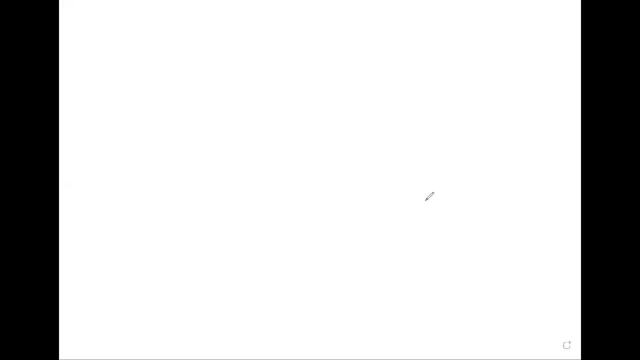 So you pay attention. one, they will look at one, a complete number, two, three, four, five, six, seven, eight, nine, 10,, 11,, 12,, 13,, 14,, 15,, 16,, 17,, 18,, 19,, 20,, 21,, 22,, 23,. 24,, 25,, 26,, 27,, 28,, 29,, 30,, 31,, 32,, 33,, 34,, 35,, 36,, 37,, 38,, 39,, 40,, 41,, 42,, 43,, 44,, 45,. 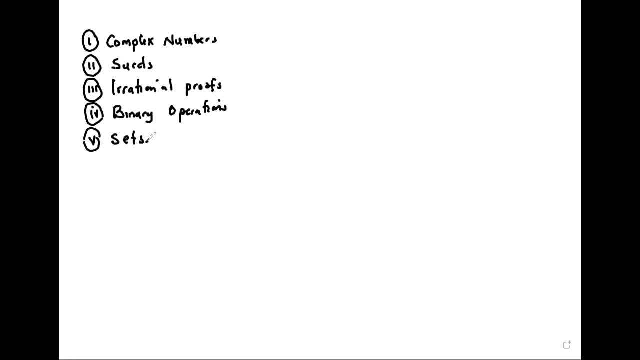 46.. Okay, so let's start. So let's start The first one. Complex. So there are so many questions on complex numbers, but the basic idea is: first thing, one should understand how to evaluate i to n power. 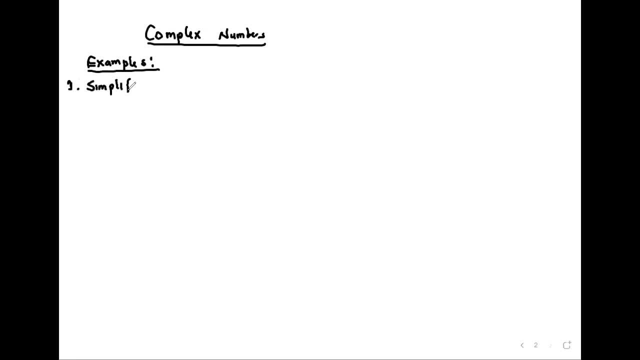 So let's simplify: A 2i power 4 minus 3i power 107, plus 7i power 13, minus 3i power 13.. So are we able to reduce regardless of how big the power of i is? maybe let's say plus. 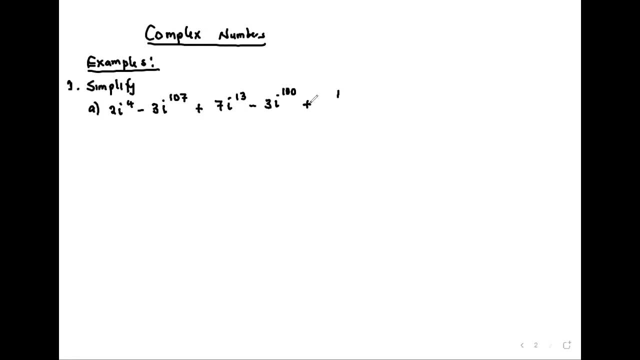 4 over i to the power 77.. Are we able to simplify such An expression? So we understand that i is equal to the square root of negative 1.. That's the first thing. The second thing: if you square i, then you remain with negative 1 on the other side. 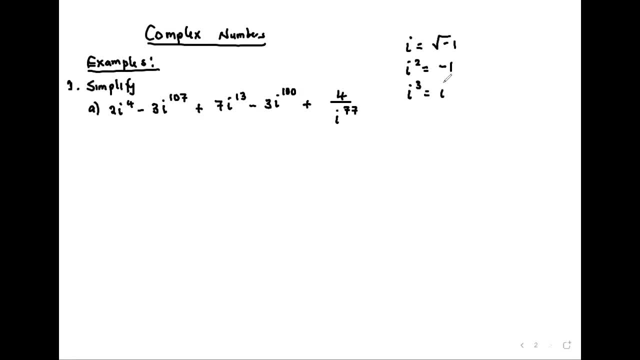 So if we do i to the power 3, you have i squared multiplied by i. But i squared is negative 1.. Multiplied by i, you get negative i. Then i4 is going to be i squared by i squared, which is negative 1, by negative 1, which is 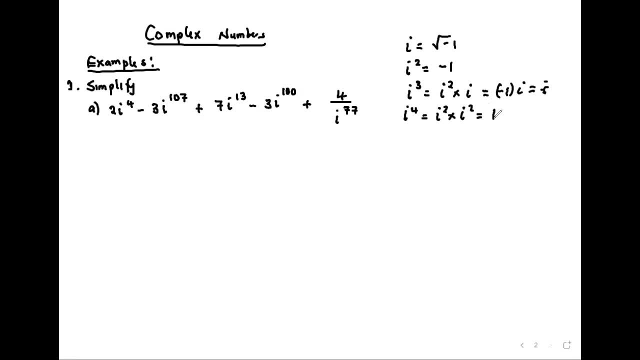 plus 2.. What? So? that's enough. Maybe we check again. what is i5?? It is the i4 times i, which is just i, because i4 is 1.. So you could keep going. So let's see how we apply that on all this. 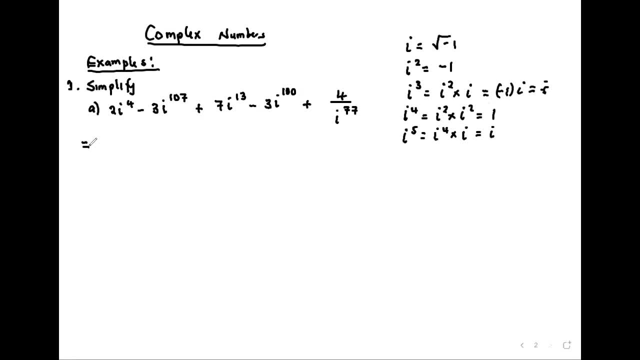 The first one is 2i4.. It does seem that i4 is 1.. So write 2 times 1,, which is just 2, minus. What about i to the power of 0.7?? i to the power of 0.7 can be written as i to the power of 0.6. 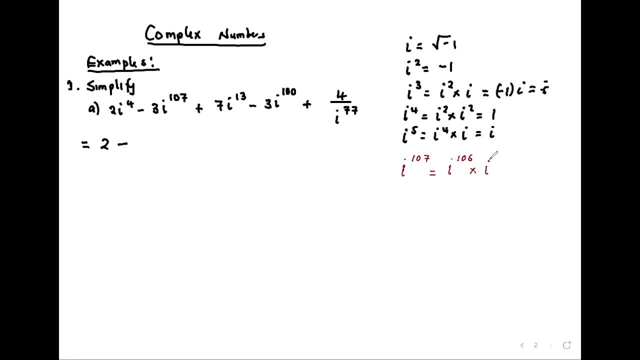 multiplied by i, That's the same thing as 106.. Like that, Now 106 can be written as i squared. Okay, I'm dividing. now I divide 106 divided by 2. So I'll have 53 here times i. 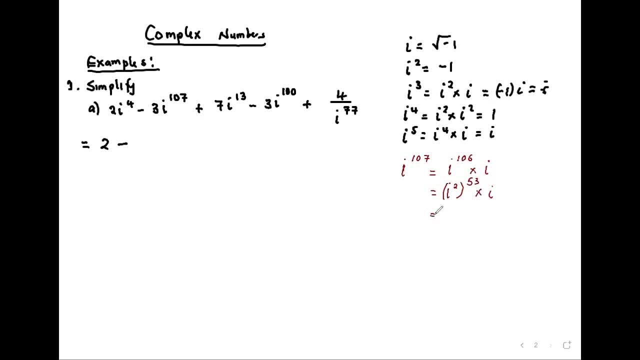 That's 53. When you multiply it by 2, I get 106, then plus 1,, 107.. So I have to remove it. Now i squared is negative 1.. Negative 1 for 53 times i. 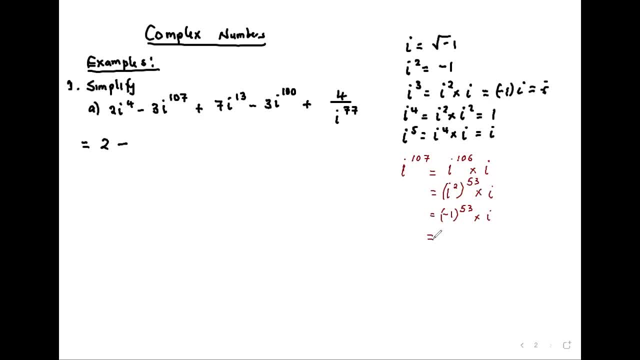 Negative 1 to any odd power remains negative 1 times i negative i. So here we go, We have 3.. We have 3 multiplied by negative i Plus 7i. What is i power 13?? Another way is i power 13.. 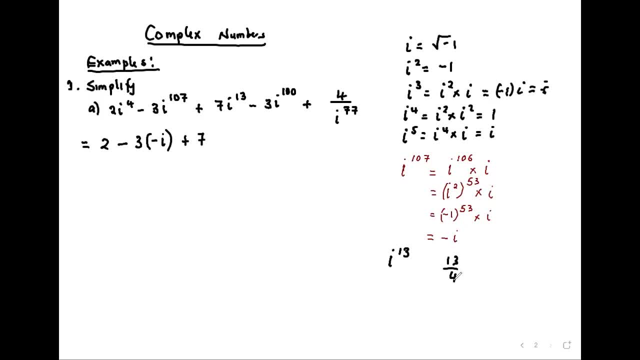 Well, you could get 13 and divide it by 4.. 13 into 4.. 13 into 4 is 3, remainder 1.. So then I just get the remainder. So I'll say I'm dealing with i to the power 1.. 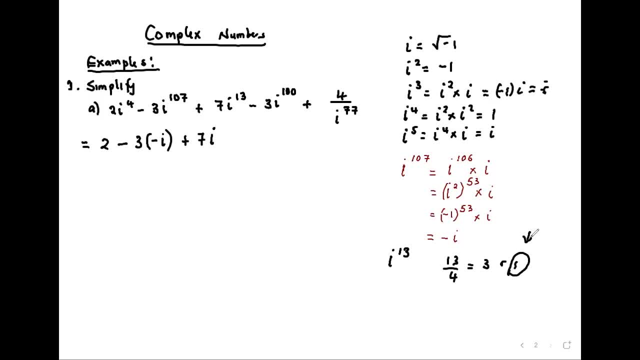 The remainder, because therefore you know, i4 is 1. So you have 1 power 3. So you can just put the i to the power 1. Minus 3, i power 100. And then divide 100 by 4 and see if the remainder 100 by 4 is 23.. 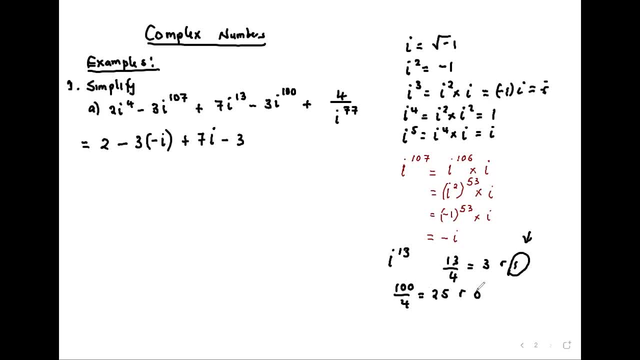 Remember 0. So it means that, as this remainder is 0.. So there we're, just at 3, because i0 is 1.. Plus 4 over i to the power 77. Again, let's divide 77, divided by 4 is equal to 1.. 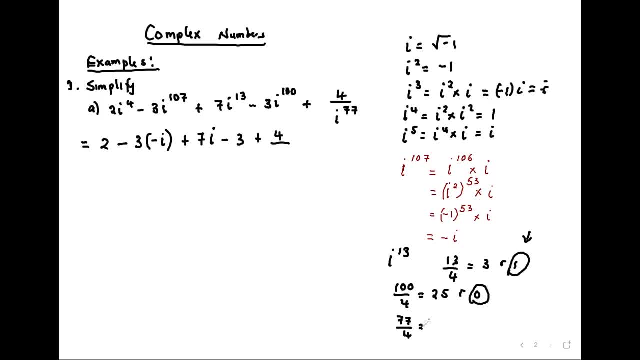 Okay, so then Remember to keep the power. Let's see then: to 5 by 4, it's 18.. So in 77, it goes in 72,, 18 times, In 76,, 19 times. 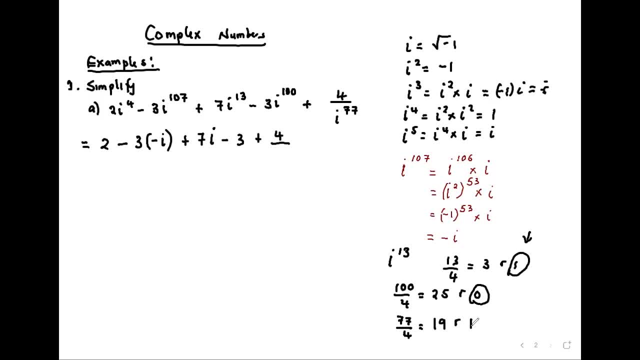 So we'll have 19,, remember 1.. So again I will have i to the power 1 in the treatment. So now we'll have 2 plus 3i plus 7i minus 3.. And then now the 4i: we'll have 4 over i, then multiplied by i. 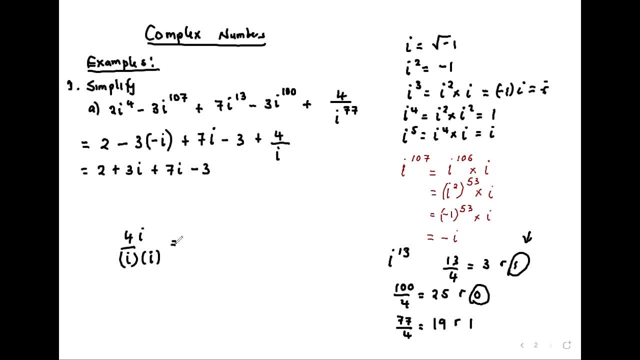 And also up by i. So now we're conjugating, So we'll get 4i over negative 1, which is negative 4i. So we'll have minus 4i. So we get 2 minus 3, that's minus 1.. 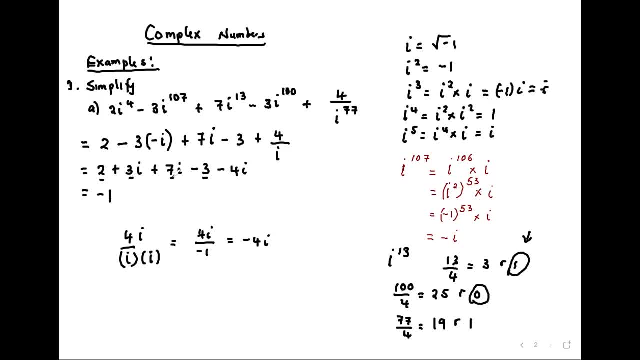 And then 3 plus 7, that's 10.. 10 minus 4, that's 6i. So this becomes after: And that's good, Okay, Okay, Any issues? Okay, Okay, That's why you are converting the. 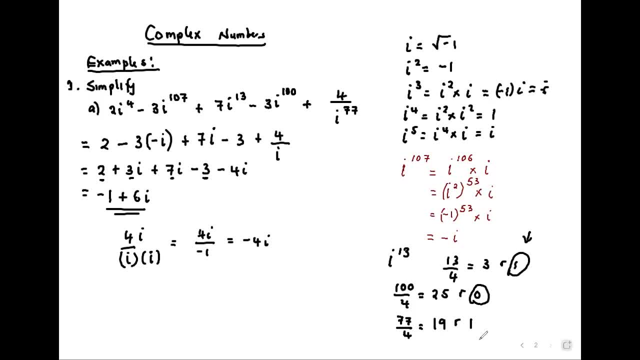 Okay, you can just repeat on the. Okay, you can just repeat on the 3i to the power 107.. Like how you ended with negative 3 brackets, negative i. So I'm saying 1 through 7 can be written as 1 through 6 plus 1.. 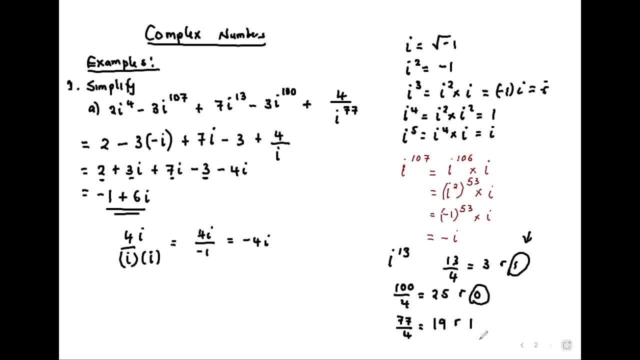 And to write 1 through 6 plus 1, we can write, since there are the powers of i, so we can have i 1 through 6 times i times 1.. Now 1 through 6 is the same thing as 2 times 53.. 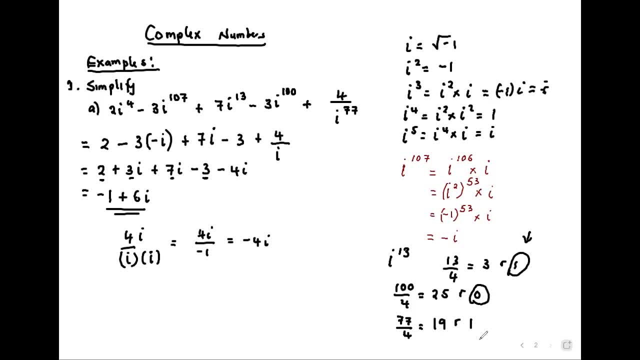 So we can have: i 1 through 6 times i times 1.. Now, 1 through 6 is the same thing as 2 times 53. So we can separate. so we can separate, we have 2 and 53.. 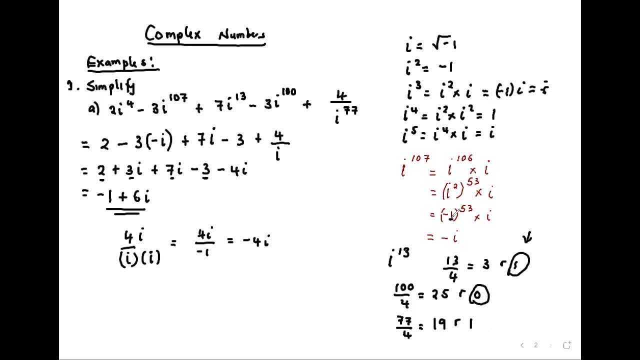 But i squared is negative 1.. So negative 1 plus 53, it gives us negative. 1 plus 53 is an odd number And then times i. so we just end up having the negative i. Then we take and substitute where there's i, 1,, 0,, 7.. 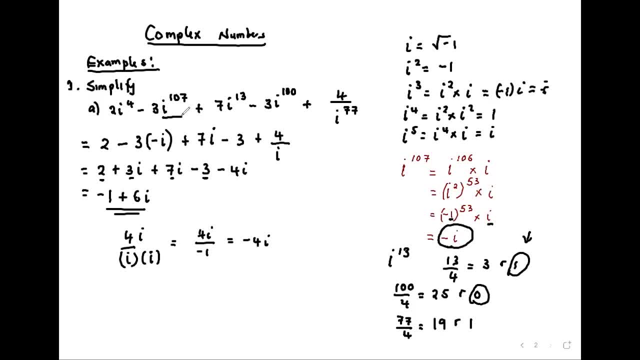 Because some of those are in. it's only the power of i and not the i, So we just end up having the negative i. Then we take and substitute where there's i- 1,, 0, 7.. uh, i wanted to ask what, if you just use the concept of saying if the power is? 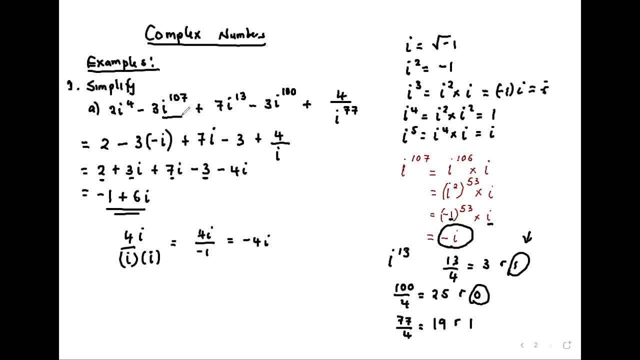 meaning that you get the actual number. i don't know if you huh, if the power is even- hey, let's say 107- then you not say that, if where are these ones? or seven, if i just get hundred. meaning that the answer that i'll get is: 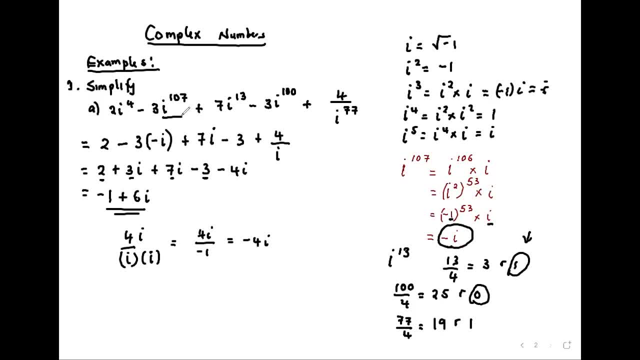 one, huh, then you also get six. you know that six again, it's even i'll get one for me- that the answer there is going to be. so the concept of- because it's evening, i'll get that, what we know is even gives us either a positive one or a negative one, and then, odd, gives us either positive i or negative i. 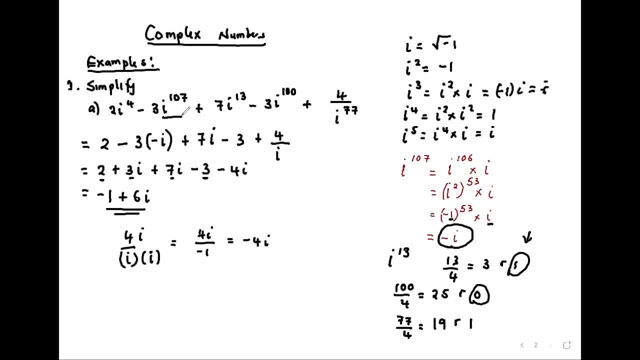 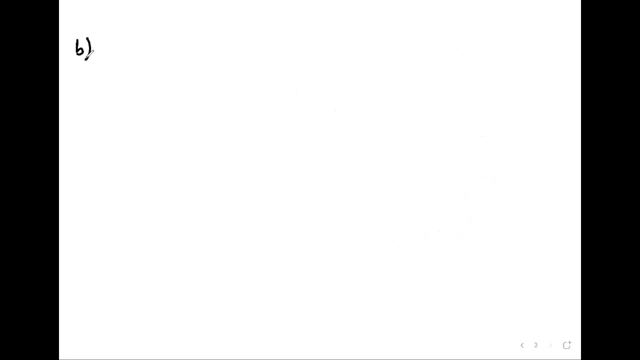 so that's when the checking comes in, because we have two options, right, thank you. so okay, another question is um, b, um. let's z1 be equal to three minus i said to be equal to one over one minus two. i are three z three will be equal to. 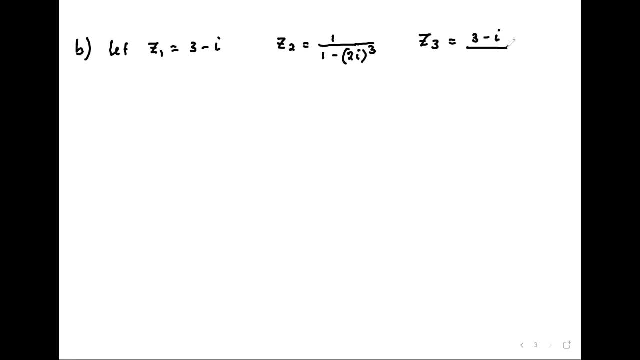 three minus i over two plus, i find find one z two. i mean z one absolute, and then three: two is equal to z one over three. z 1 bar. z1 bar. three z1 bar, so that z 1 bar ач one z3 divided by, by z one and five z two over. 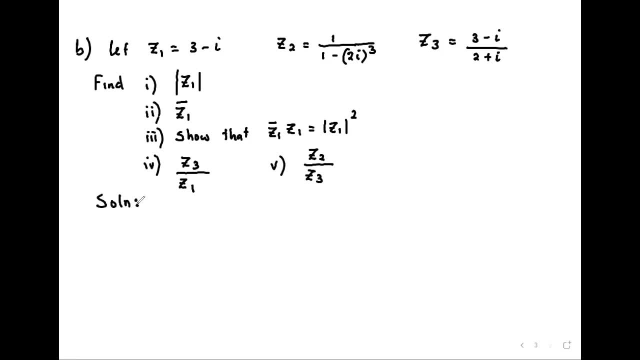 solution. so to define the absence, if, if z is x plus i, y, the absolute of z is defined as the square root of x squared plus y square. that is the definition. so our y, the absolute of z one, is going to be the square root of with square three plus we spend at the point. 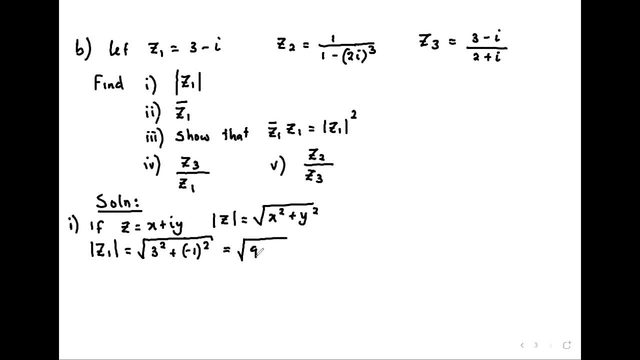 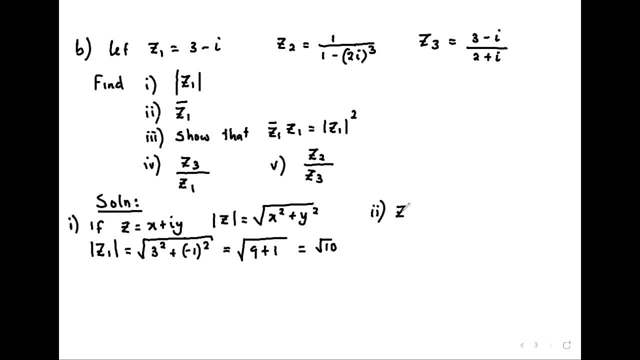 and then two to get z one bar. you get the conjugate of z one. so since that one is three minus i, z one bar is three plus i. and then part three show that z one bar multiplied by z one is the absolute of z one spread. 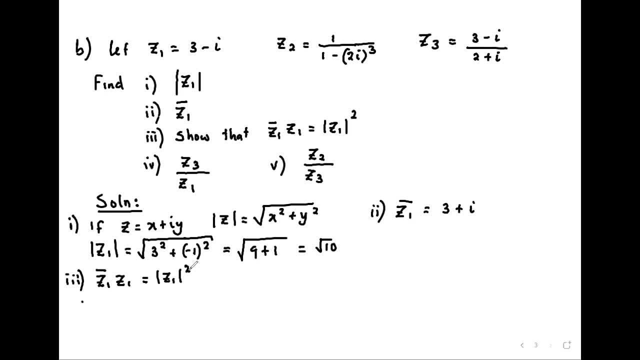 so well, we have already found the right hand side. we have found z one, but i mean z one. up to now we just want to spread. so i get in the root of ten and then have the spread. so get ten, and then we also get the left hand side, which is z one bar multiplied by z one. now z one by is three plus i. 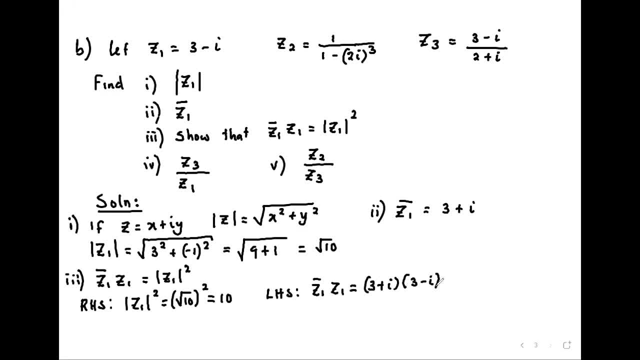 and z1 is 3 minus i. So we multiply 3 by 3, 9, minus 3i plus 3i. i times i is negative 1, and the negative is negative 1,, which gives us 10.. 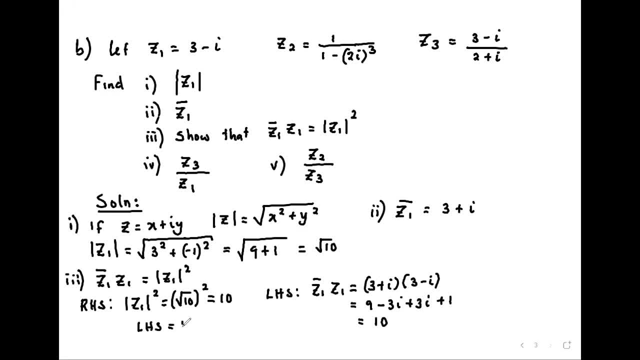 As we can see, left-hand side is equal to right-hand side. So like that, Like that, Like that, Any questions, Any questions, No questions, Good. Next. So I can repeat, on the z bar. So z bar is the conjugate of the z. 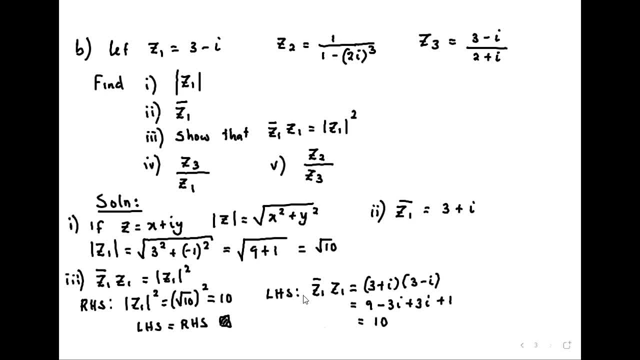 So you change the sign of the marginal part, The number that has i, you change its sign. If it was, if it was negative, you put plus. If it was plus, you put negative. The other one, you leave it like this: 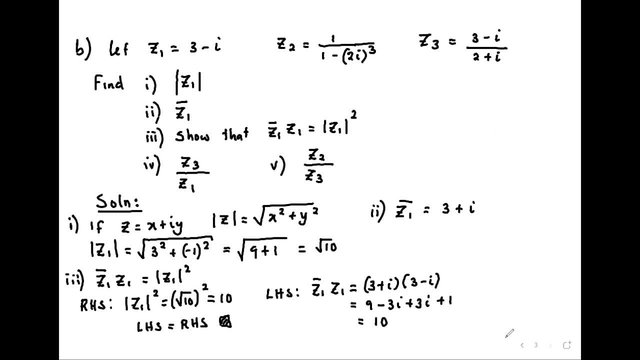 Okay, Then what about z3 over z1? So let's do it from here: z3 over z1.. That is z3, is 3 minus i over 2 plus i. you divide by z1.. That is 3 minus i. 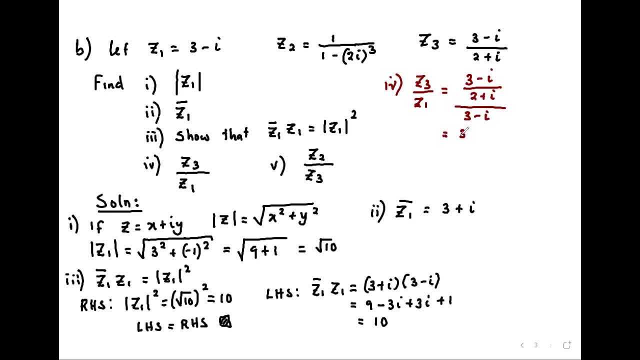 So this is: you can write this as 3 minus i over 2 plus i, divided by 3 minus i over i. So you can write it like this: over 2 plus i over 2 plus i. 1, which can be written as 3 minus i over 2 plus i, multiplied by 1 over 3 minus i. 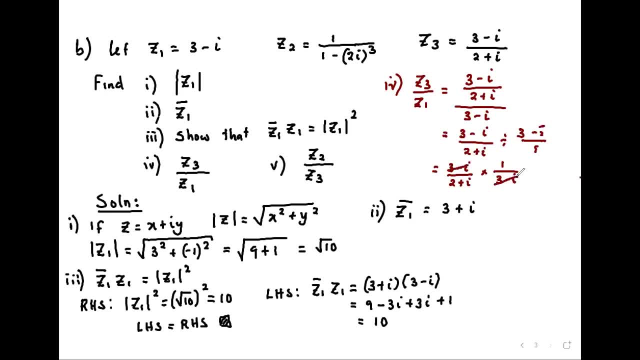 so you can see that this and this will cancel. so you end up having 1 over 2 plus i. and then you conjugate it, so you multiply 1 by 2 minus i over 2 plus i, multiplied by 2 minus i, so you have 2 minus i over 4 plus 1. 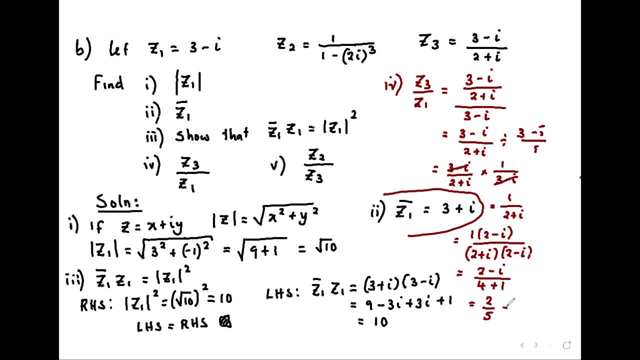 giving us 2 over 5 minus i over 5, the 4 plus 1 is what you get. when you expand the 2 plus i by 2 minus i over 5, minus i over 5 plus 1, squared times six, that gives you 4 plus i divided by 2. 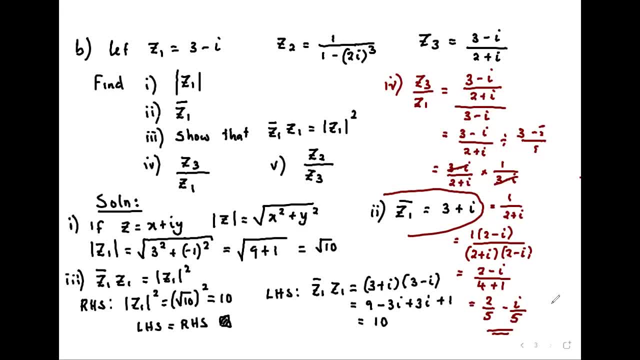 5, and now these two smaller numbers together are £ surround. Next is Z2 over Z3 back. Let me clear this part so that I can go into code. So file Z2 over Z3. It will be: Z2 is 1 over 1, minus what is 2 to the power 3?. 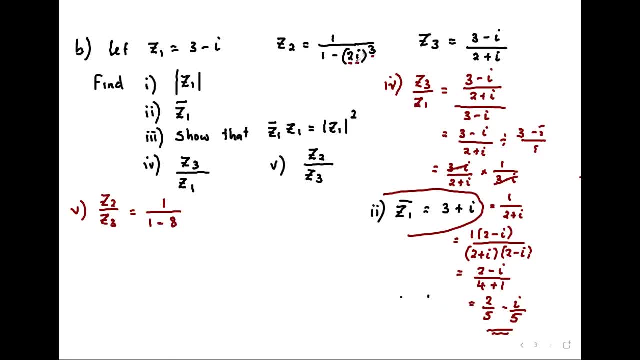 It's 8.. And the i to the power 3 is negative. i It's negative. i It's negative. i For this, divided by Z3, which is 3 minus i, Which is 3 minus 3.. Minus i over 2 plus i. 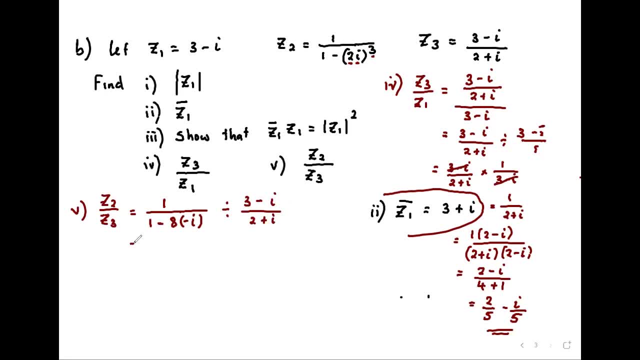 Okay, Then we simplify. The other one is 1 over 1 plus 8i. Now we can use multiplication 2 plus i over 3 minus i, Common denominator 1 plus 8i By 3 minus i over 2 plus i. 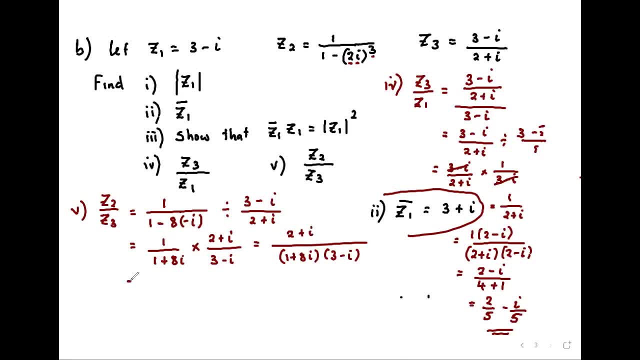 And then you do the expansion, So you have 2 plus i over 3, minus i plus 4i. What do you get? So you get H equal 2 plus i, And then plus H, Which is 2 plus i over 11 plus 23 i. 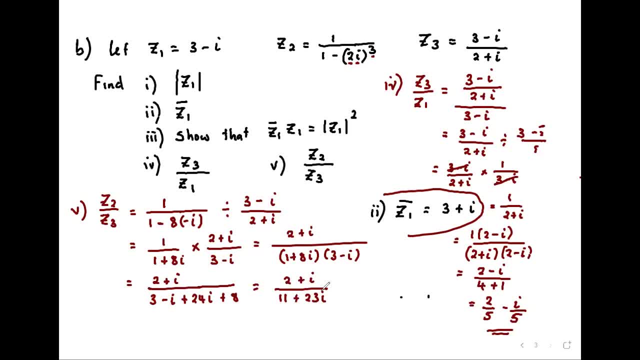 Then from there, now you can you get. so you multiply by 11 minus 23 i and 3.. That's right, You multiply Like You have done. You have done 1 minus 23 a. 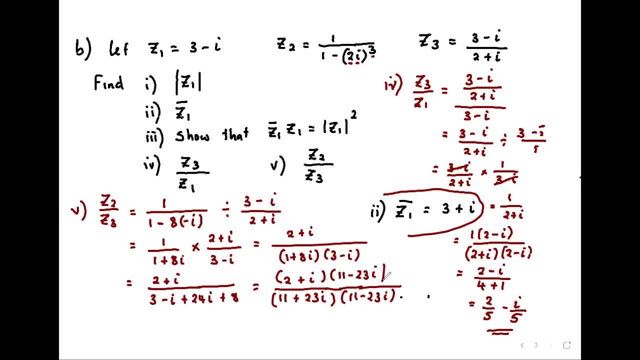 and then you get the solution. now, this is what we call conjugation, so the skill that i'm teaching you here is be clear. uh, so you need to know how to communicate. i think that's much all about complex. the other type is. the other type is, i think, one more time. 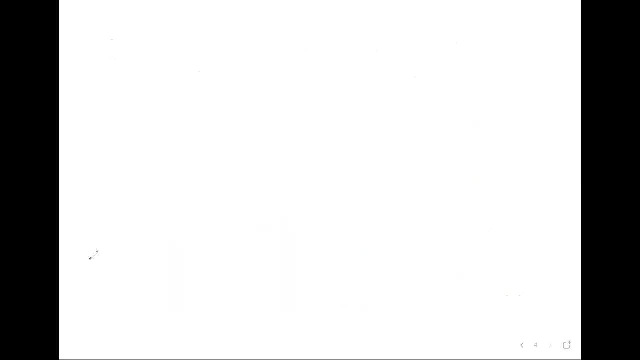 the other type is this, one that is three, an equation: find x and y. if i'm given x plus i, y over, maybe three minus five i is equal to, is it one plus two, i plus three over twenty, one minus i? and then you're asked to find x and y, what you do. 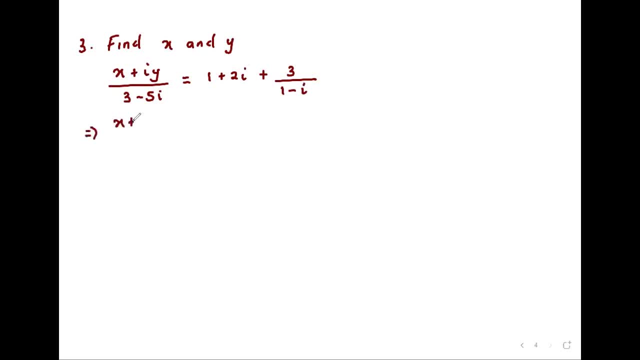 are you. you have x plus i y over 3 minus 5 i is equal to 1 plus 2 i plus 3, 1 plus i, one plus i over one minus i, one plus i. so you're going to get. so you get- x plus i y. 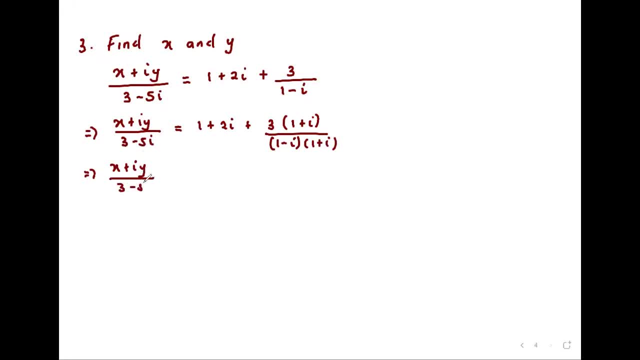 over three minus five, i is equal to one plus two. i plus three plus three. i over this will give us one plus two. i mean one plus one, which is a two. so i'll put a two here and a two left and then now cross, multiply, so we multiply throughout by. 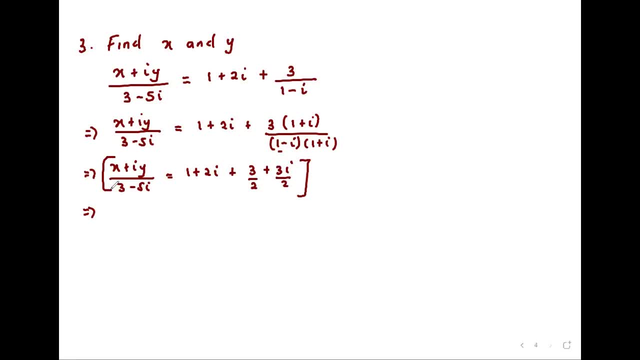 by three minus five i on the left, we remain with x plus i, y on the right, we'll have the product to one plus three over two plus two, i plus three. i over two. multiplied by three minus five, i. that is one plus three over two, that will be five over two. 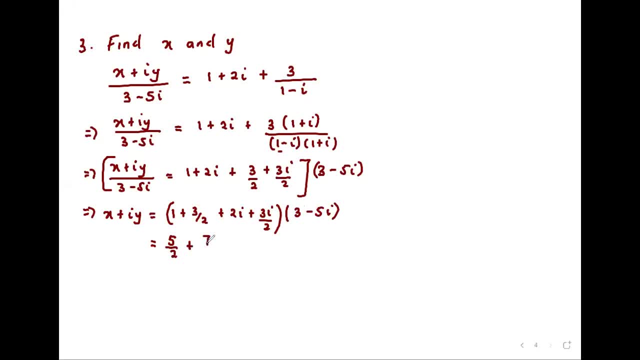 plus seven, i over two. when we add the two. if you put the one there and then this, you multiply by three minus five, i giving us fifteen over two minus 25. i over two plus 21. i over two minus 35. i squared over two. so the i squared makes it. 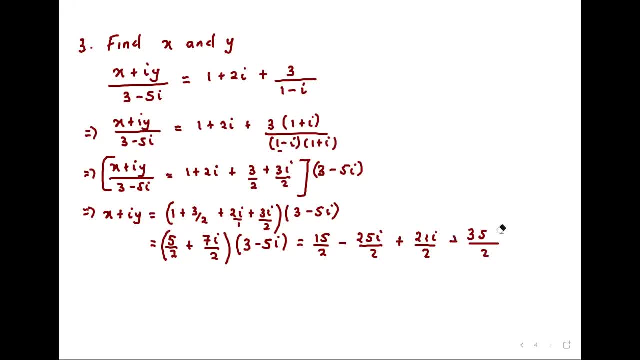 minus, which gives a positive here. then now we put the right hand together, so we have 15 plus 35. that gives us this 50. So we have 50 over two minus 25, at last 21, that will be minus four, i over two. 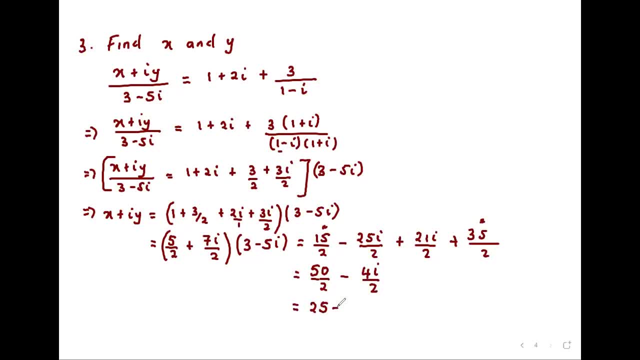 so we have 25 minus two i. this is equal to x plus i one. so x is 25, y is minus two. like that soon. So that's so much about complex. There's no question on complex. that can come to supply test Qualification you first add. 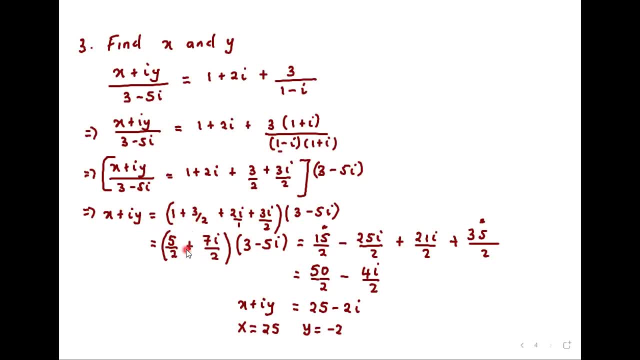 when you first add and then you multiply. now, 5 over 2 times 3, you get 5 times 3, which is 15 over 2.. 5 over 2 times 5, you get 25 over 2.. 7 over 2 times 3, you get 12 over 2..